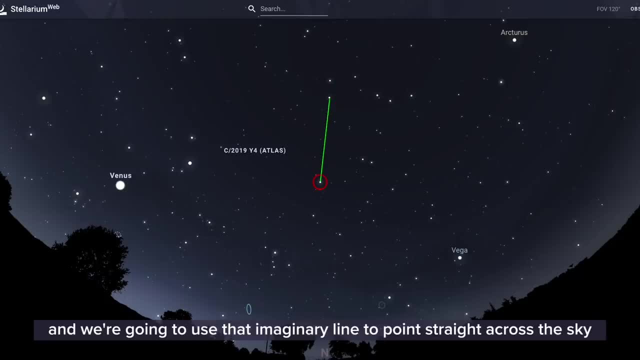 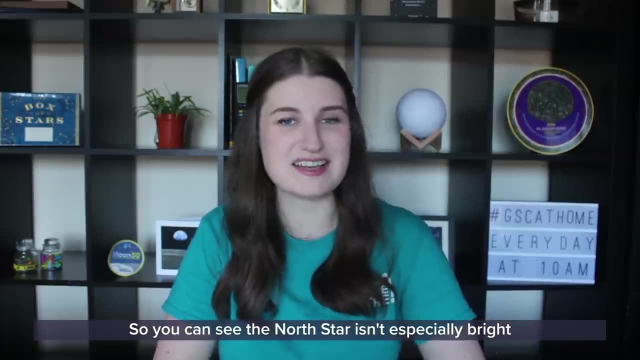 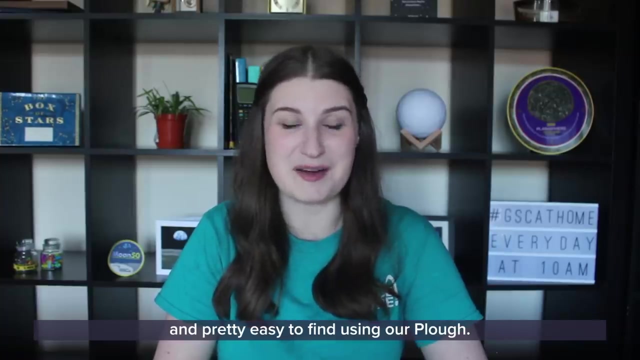 we're going to use that imaginary line to point straight across the sky and they go straight to the North Star. So you can see the North Star isn't especially bright, but it is still bright enough to spot in a city and pretty easy to find using our plough. And now you will never get lost again because the 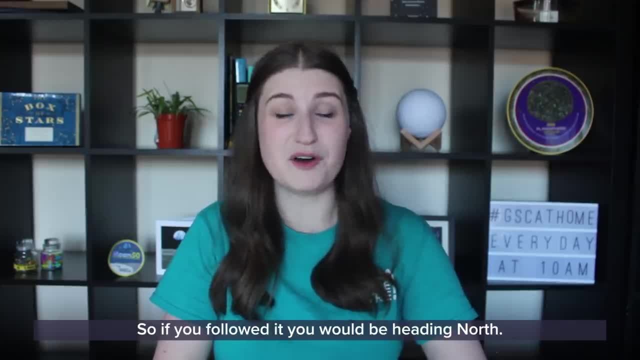 North Star is a very bright star. It's a very bright star. It's a very bright star. The North Star is right above the North Pole, so if you followed it, you would be heading at North. You can point to the North Star. drop your hand to the horizon. and you know that is where North is. If it's to your right, you're travelling west. if it's to your left, you're travelling east, and if it's behind you, you're travelling south. If you wanted to measure the angle between the North Star, 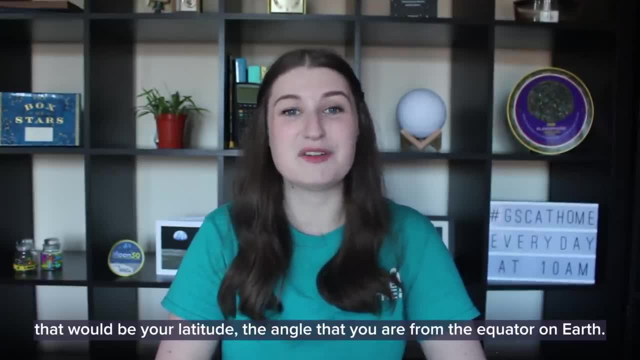 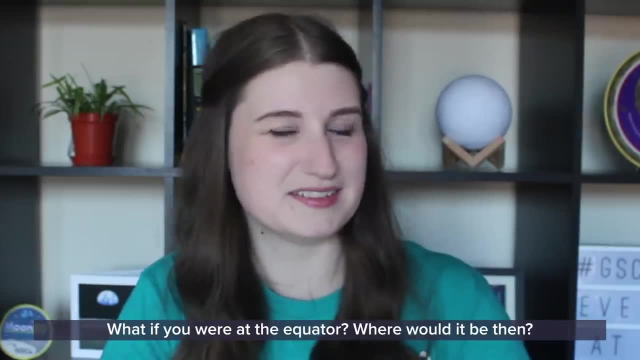 and the horizon. that would be your latitude, the angle that you are from the equator on Earth. If you were at the North Star, you would be at the North Pole. If you were at the North Pole, where do you think the North Star would be? What if? 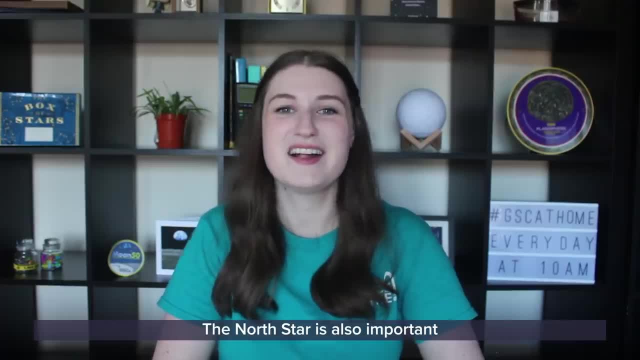 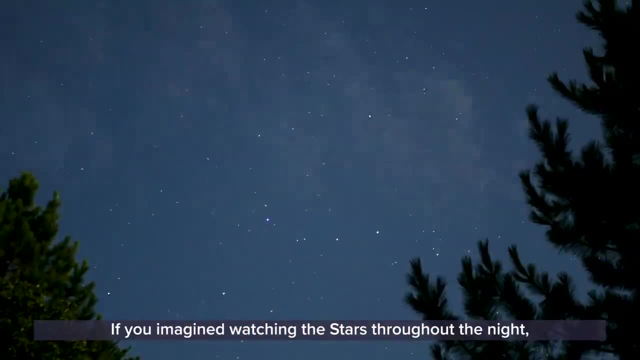 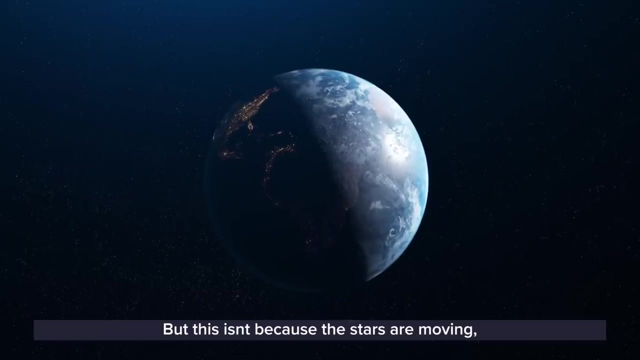 you were at the equator, Where would it be then? The North Star is also important because it's the only star that stays in the same place. If you imagined watching the stars throughout the night, it would start to look like they would move across the sky. But this isn't because the stars are moving. it's 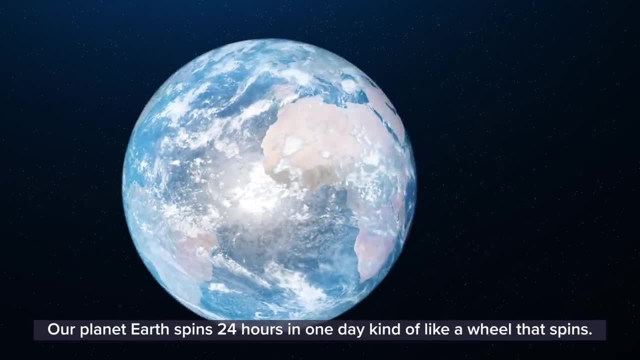 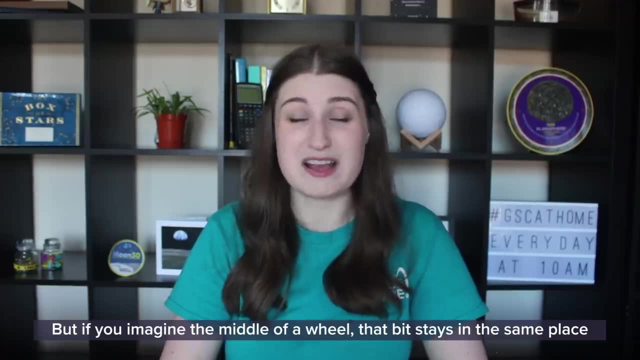 because we're moving. Our planet Earth spins 24 hours in one day, kind of like a wheel that spins. But if you imagine the middle of a wheel, that bit stays in the same place and that is just like our North Star. It's above our North. 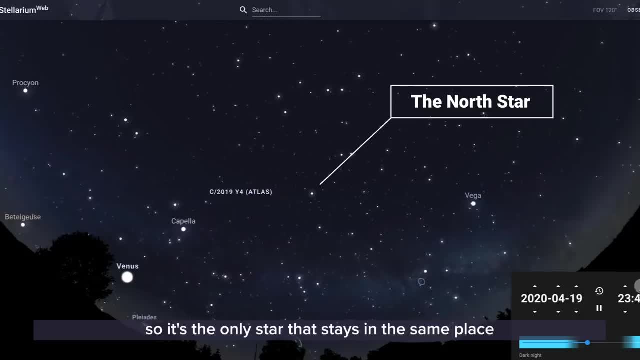 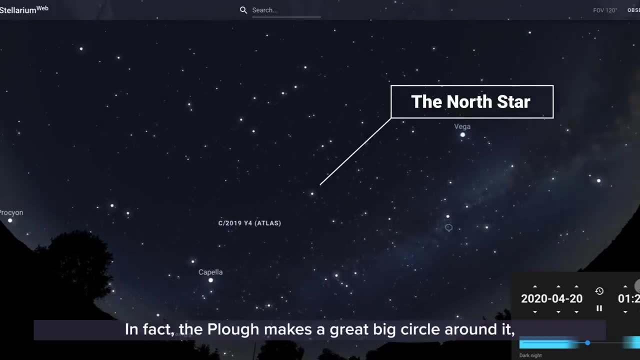 Pole that our planet spins around, so it's the only star that stays in the same place, and all the other stars look like they go around it, just like you can see here. In fact, the plough makes a great big circle around it, but you can. 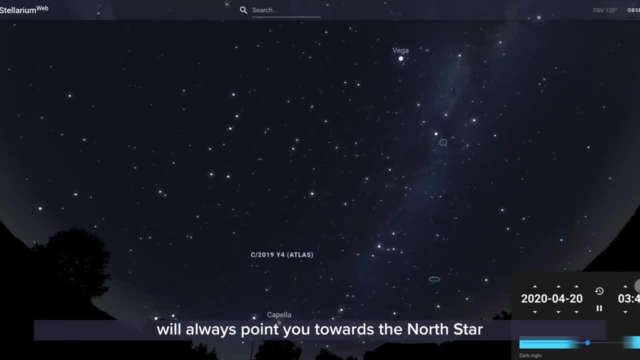 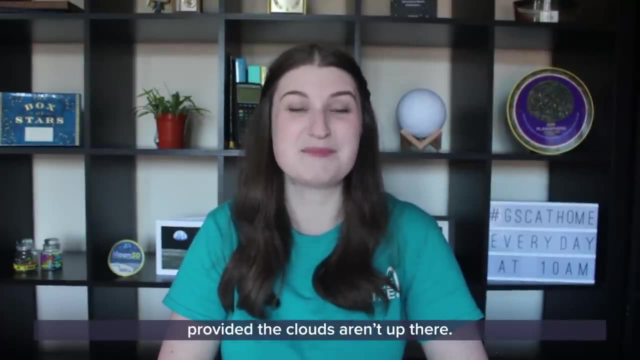 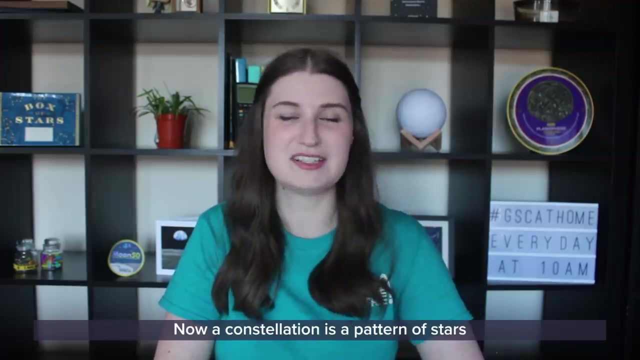 see that, no matter what, those pointer stars will always point you towards the star, and from the UK we can do that any night of the year, any time of the night, provided the clouds aren't up there. Another common mistake is that the plough is a constellation. Now, a constellation is a pattern of stars that is recognized. 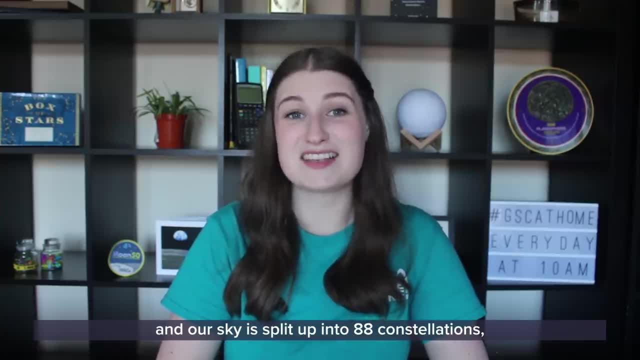 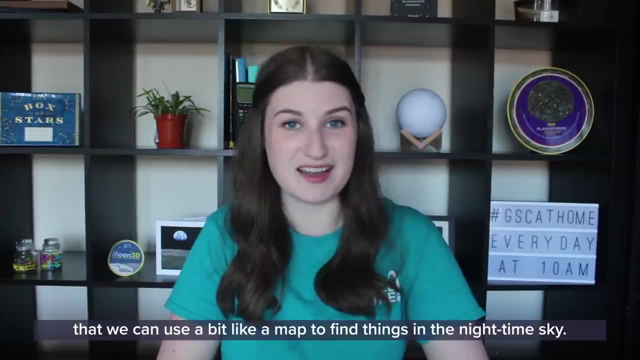 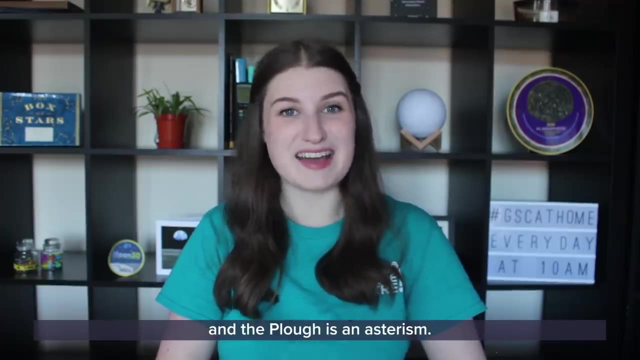 by the International Astronomical Union and our sky is split up into 88 constellations that we can use a bit like a map to find things in the nighttime sky. Any shape that isn't a constellation that we make is called an asterism and the plough is an asterism.